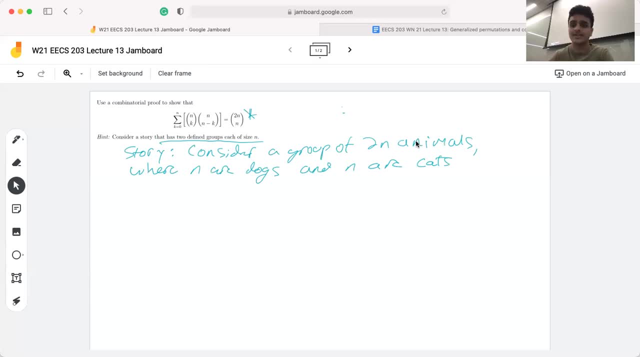 So we're going to try to explain how the left-hand side counts that and how the right-hand side counts that. So between the two, the right-hand side looks a little bit simpler, So let's start with that. So two N choose N. Well, the way we can think of this, 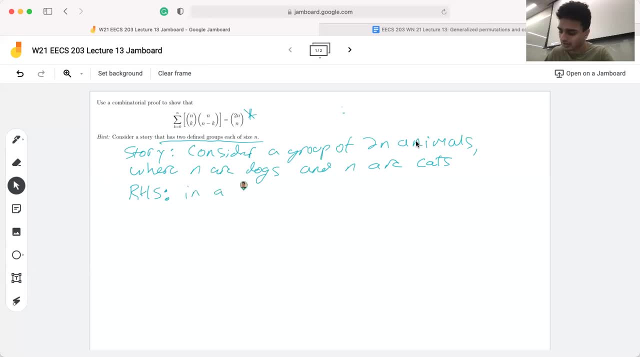 is that in a group of two N animals. so in a group of two N animals, N of which are cats and N are dogs, let's pick N to form a committee. So one interesting thing to note is that, in the context of this specific proof, 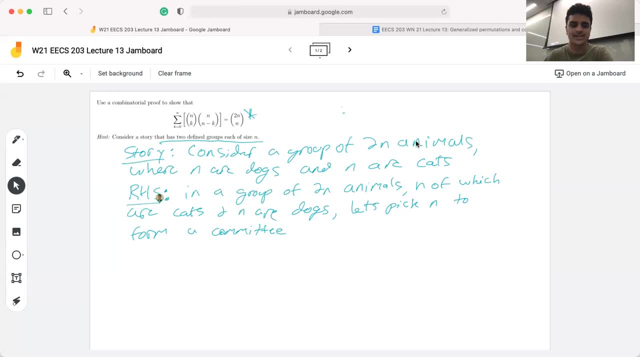 our story and our right-hand side were more or less identical, And this is something that you may or may not see, And a lot of the times, with the combinatorial proofs, it is the case that your story is pretty similar to one of the sides, but I wouldn't expect that every time. 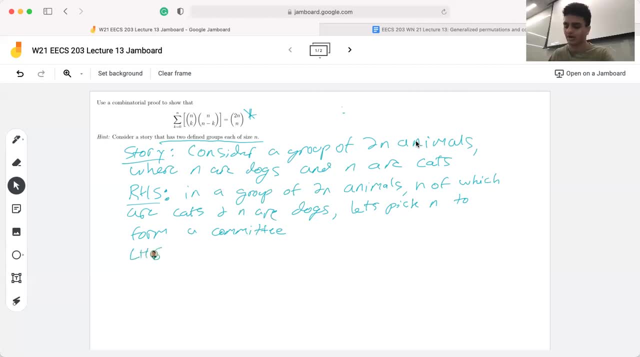 But now, moving on to our left-hand side, which is a little more complex, A lot of the times when we start with summations, we're going to start with a group of two N, So we're going to start with a. It's kind of hard to conceptualize, So what I like to do is kind of break it up right. 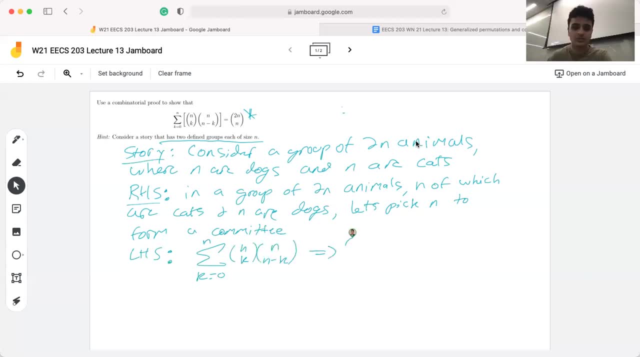 So what's actually going on here? Well, the first term would be: K equals zero, N choose zero times, N choose N plus N choose one Right. So one way we can think about this is that we're almost addressing it by cases. 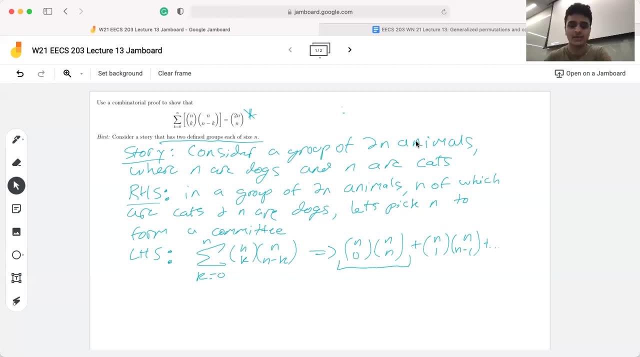 which is a lot of the time. What's happening in summation? So in this case, what we're doing is we're saying: okay, pick zero from the first group. So we're saying pick zero from the first group And let's say: 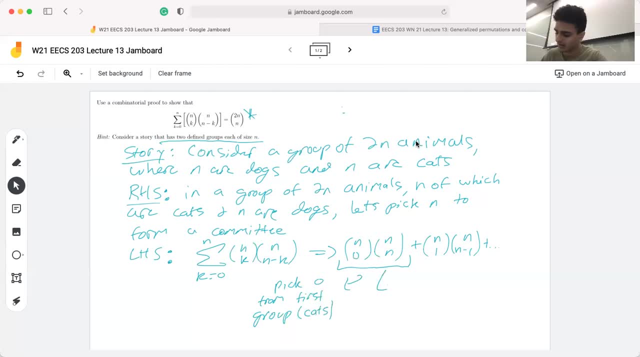 that first group is the cats. And then the second case. we're saying, okay, pick N from second group And that would be the dogs. And essentially what's happening here high level would be is that if we split up all the possible, 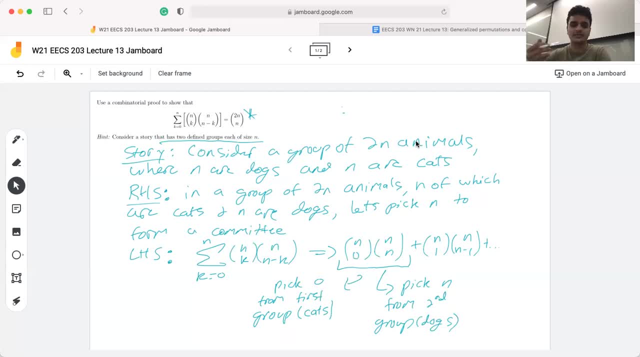 the selections in the cases. So if we're trying to pick N animals at any given point, we can pick K dogs and then N minus K cats And in total that would give us our group of N. So that's essentially what the left-hand side is counting. So now writing it a little more formally: 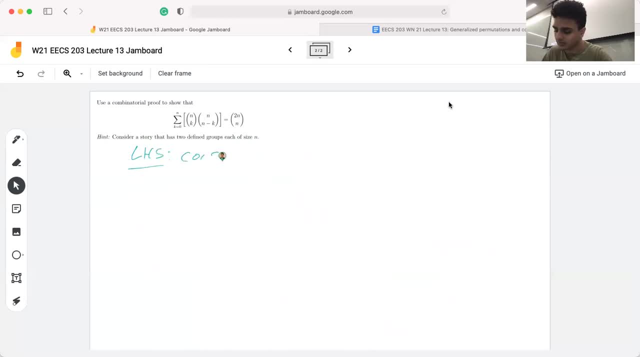 we're going to say our left-hand side is: consider all cases where we pick N. So we're going to pick K cats and N minus K dogs, And essentially the sum of those, so K plus N minus K, is going to give us N. 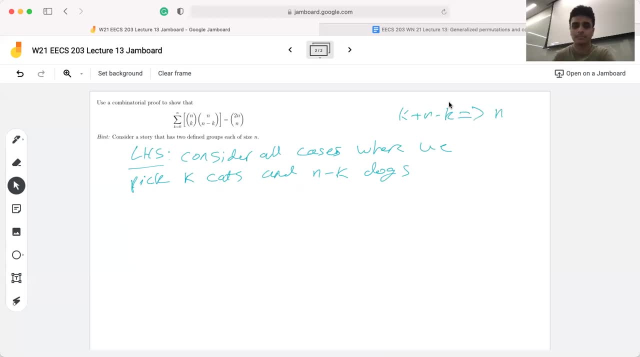 And that tells us that we're still picking a group of size N. So if we consider all the cases where we pick K cats and N minus K dogs, starting off that would mean, okay, well, let's pick zero and one. So in this first case we're saying, okay, pick zero cat, or pick zero cats. 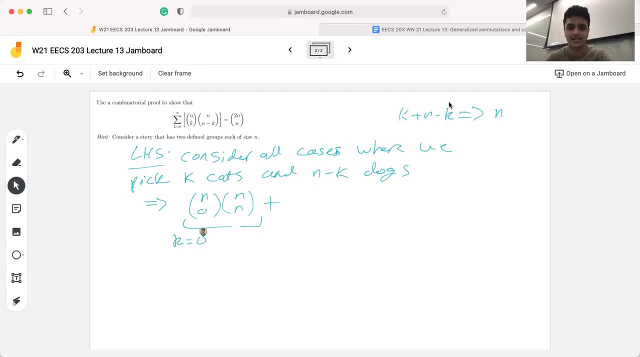 So K is equal to zero, and then pick N minus K, which would be N dogs. We're saying, okay, now let's pick one cat and N minus K dogs, And we're going to keep on adding those terms until we get N choose N times N choose zero, And this would be your K. 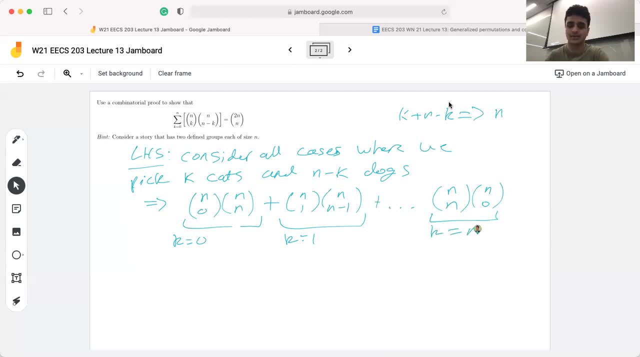 is equal to N case, And that's where we're picking N cats and zero dogs. Well, this expression simplifies to: the sum from K is equal to zero to N of N, choose K and choose N minus K. So essentially, what we're saying is that the right-hand side 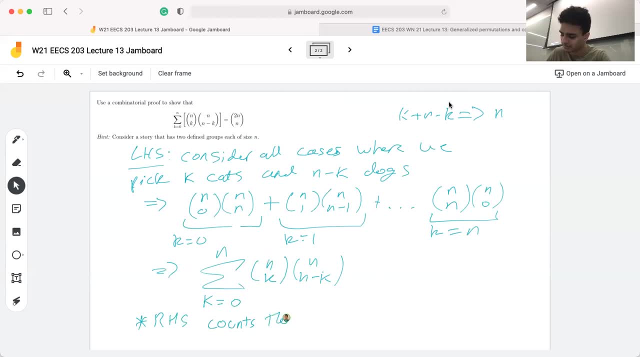 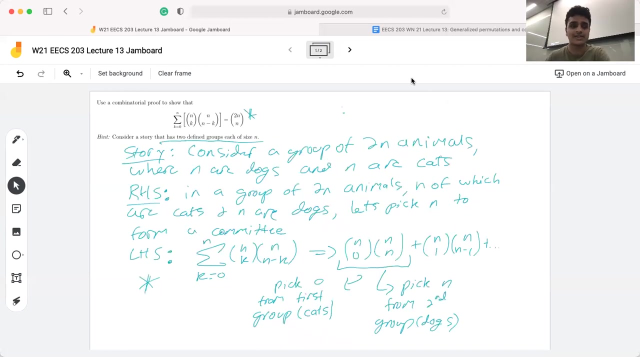 counts the number of committees by cases, And so essentially what that does is establish that, or the final part of our combinatorial proof, which is that the right-hand side and the left-hand side count the same number of things. So really quickly, just to recap what we did, so we first started by looking at the left-hand side. 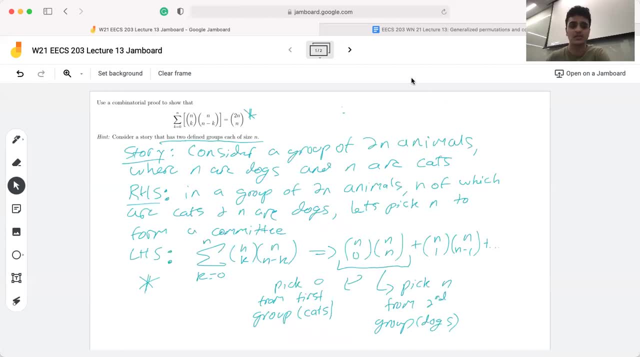 and the right-hand side, and from that kind of crafting a story which explains what's going on, in our quality, In our expression, we saw that between the two sides, the right-hand side was a little bit easier to work with, which is something you'll see a lot. And then we want to start with. 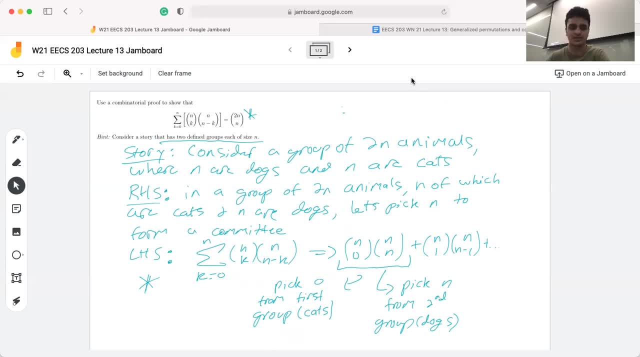 that easier side And in this case the story in the right-hand side, which we need to get the right-hand side turned out to be pretty similar. After that we looked at the other side and explained how that also counted- the same thing as the right-hand side. So essentially the 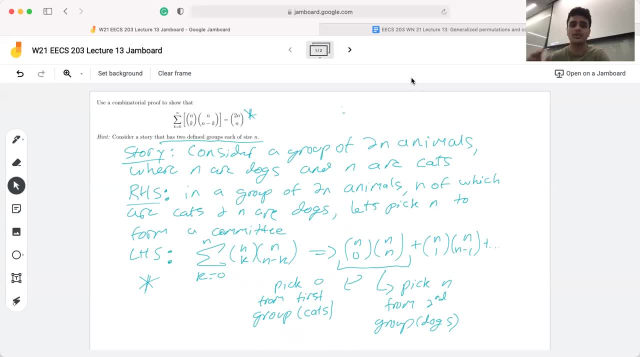 combinatorial proofs that you're going to be working with in this class can be formatted in those three main categories. Thanks for watching.